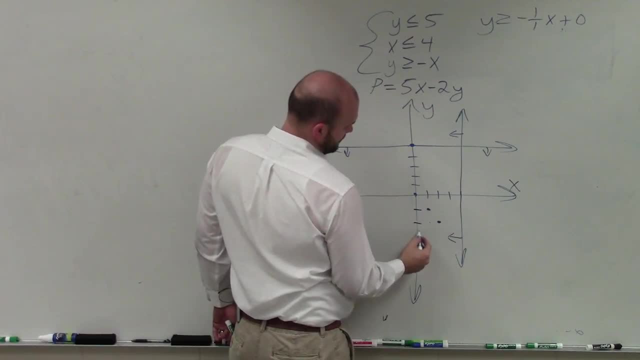 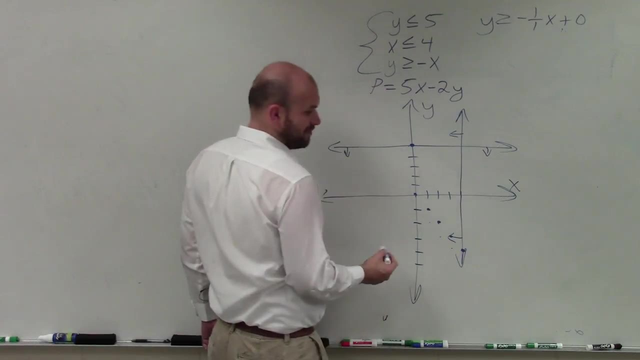 1, down, 1 over 1.. And then I go down 1 over 1, down 1 over 1.. And it's really important for us to be able to determine where those points are going to intersect, for us to obtain. 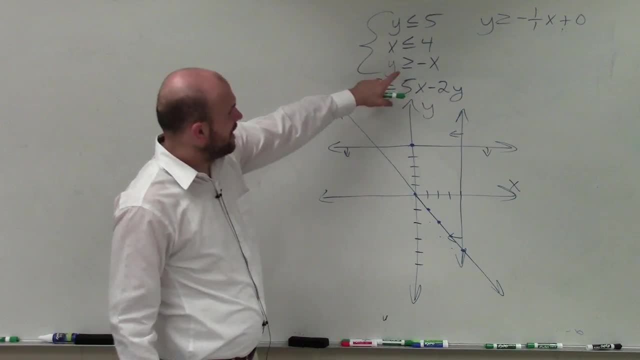 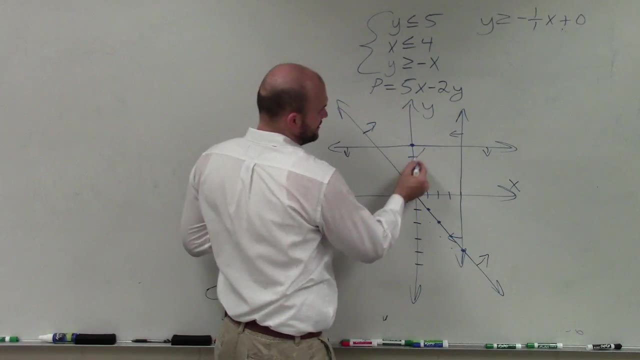 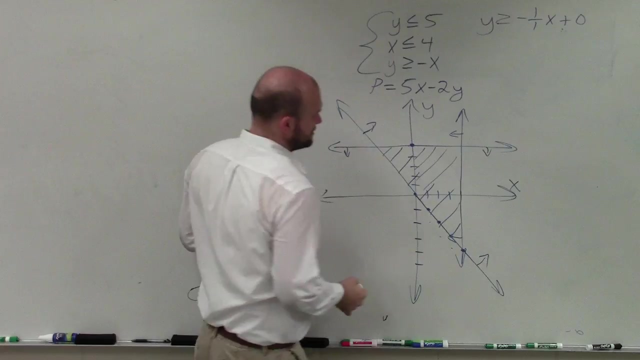 our vertices, And this is saying y is greater than negative x, So all the values that are greater than this boundary line are going to be facing up. So therefore, ladies and gentlemen, you can see that our region, our feasible region, is going to be this nice. 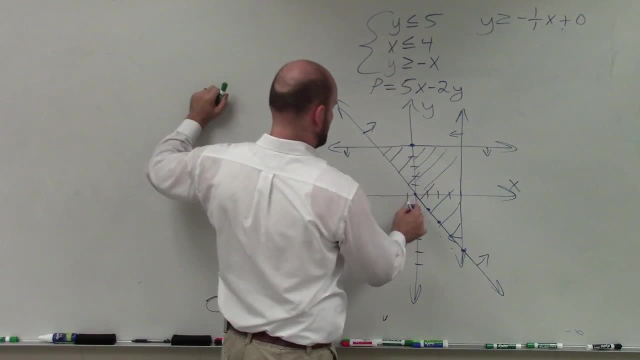 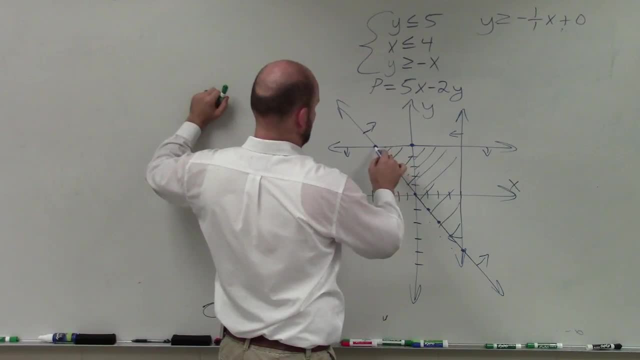 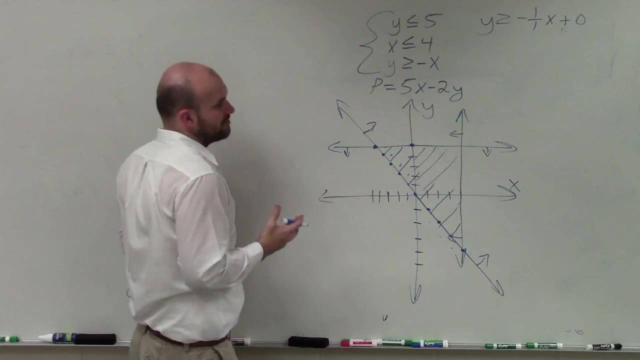 over 1, up. 1, over 1, up. 1, over 1, up 1.. So that left. that point is negative: 1, 2, 3,, 4,, 5, 4.. So now we need to be able to write. 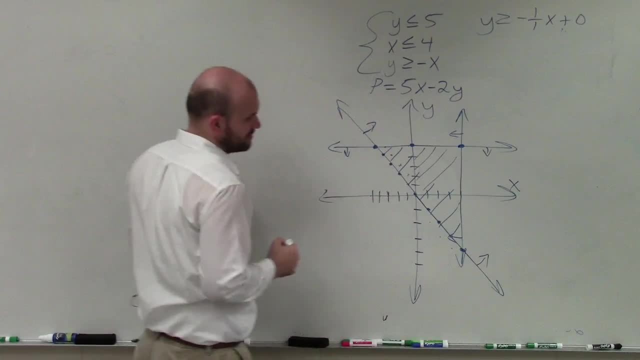 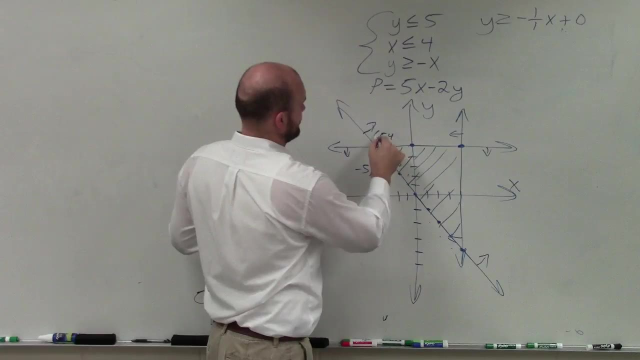 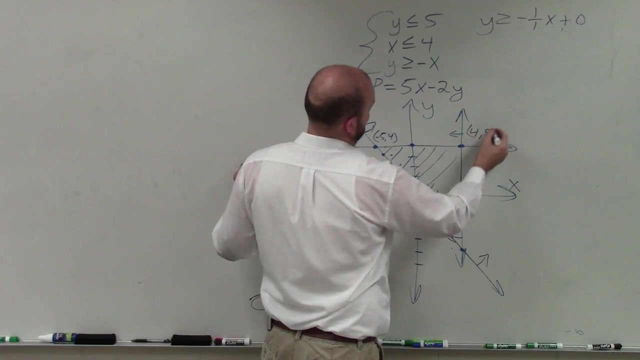 in all of the coordinate point, all these vertices where our lines intersect. So here I have negative 5, so negative 5 comma 4.. Here I have x equals 4, y equals 5. Over here I have x equals 4.. 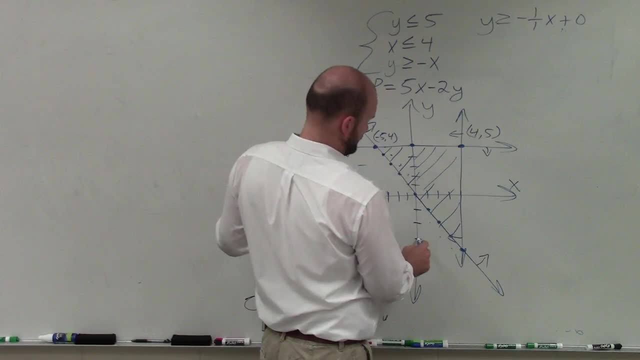 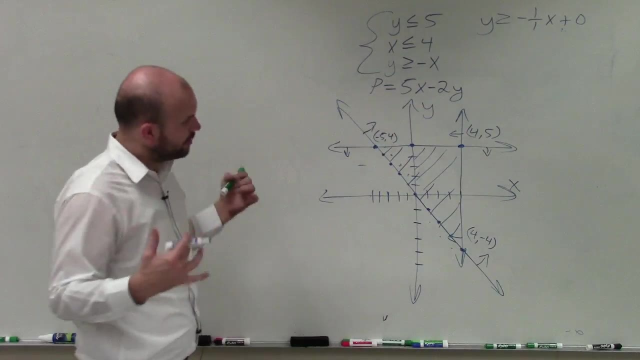 I'm sorry. x equals 4y equals 1,, 2,, 3, 4.. So 4 comma negative 4.. And those are going to be only my vertices. You can see well, why don't you use those points? 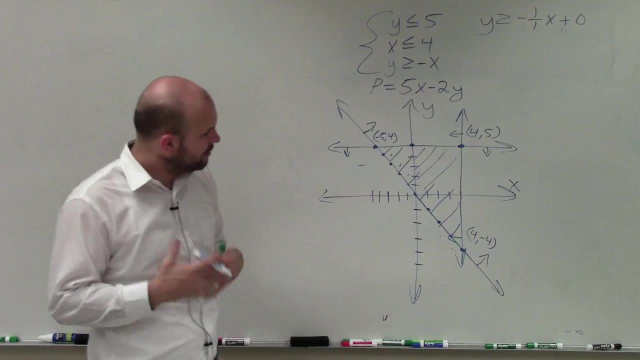 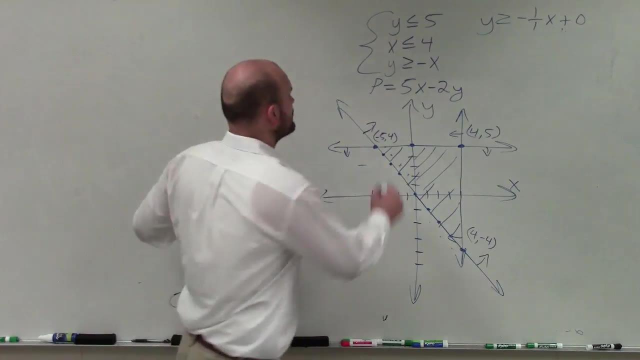 Well, that's not where two constraints met. We're only going to deal with the values where our constraints meet. Now, what we want to do is optimize our objective function. So we're going to plug in our x and y coordinates for each of our vertices and determine: 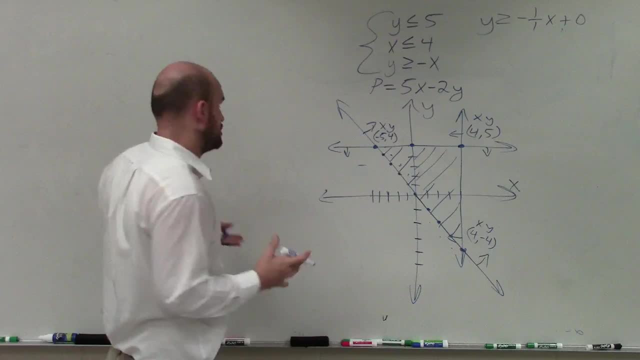 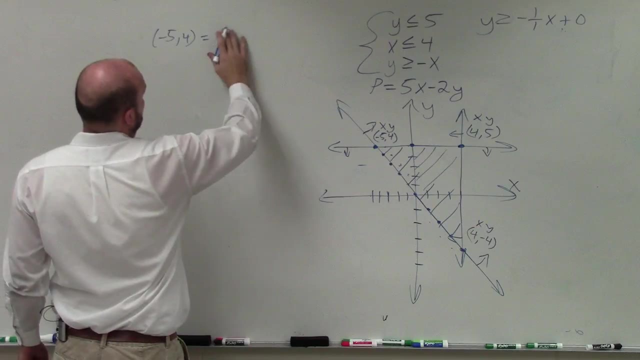 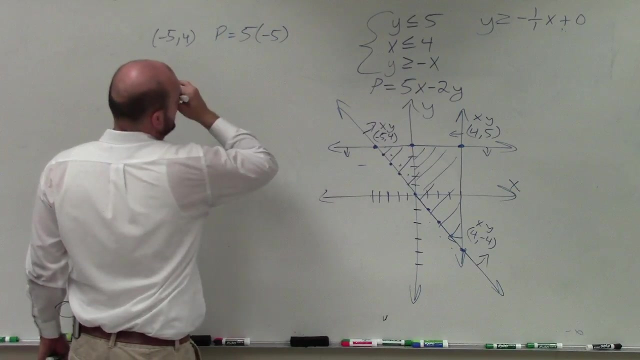 which point is going to give us our largest value. So for the first one I'll do negative 5, comma 4.. And I have that's equal to p, So that's going to be. so p is equal to 5 times negative 5.